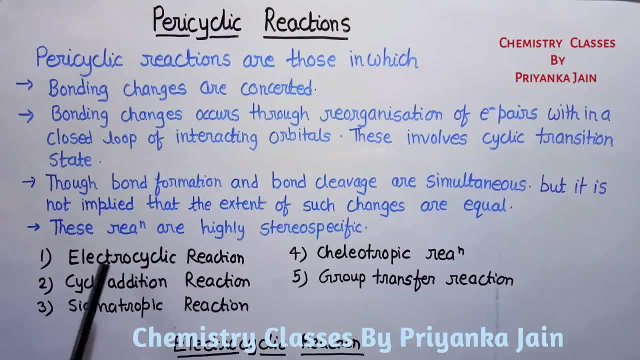 called highly stereospecific reactions, And the different types of pericyclic reactions are. there are five types of pericyclic reactions. There are five types of pericyclic reactions. There are five types of the pericyclic reaction. First is electrocyclic reaction. Another is cycloaddition. 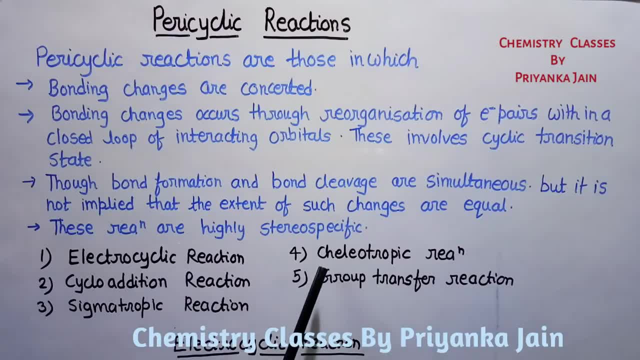 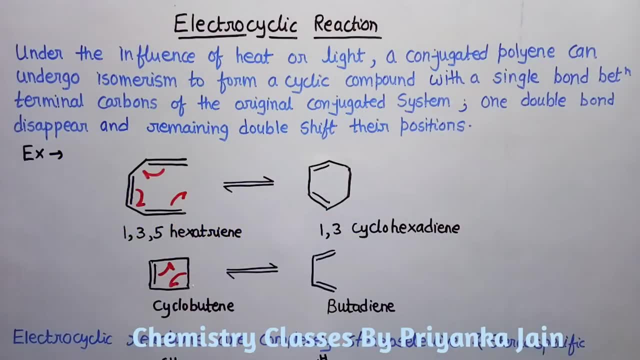 reaction. Third is sigmatropic reaction, Fourth is keliotropic reaction And fifth is the group transfer reaction. Firstly, we see the electrocyclic reactions. What are these type of reactions? Under the influence of heat or light, a conjugated polyene can undergo isomerism to form a cyclic 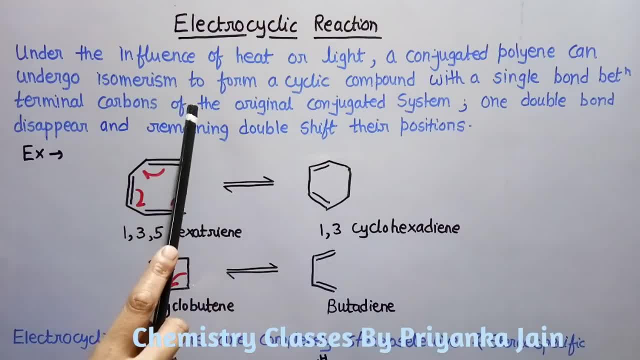 compound with a single bond between the terminal carbons and the polyene. The polyene can form a double bond between the terminal carbons and the polyene. When double bond disappears, the remaining double bond shifts their positions. What is it means? It means in an open chain conjugated polyene. It 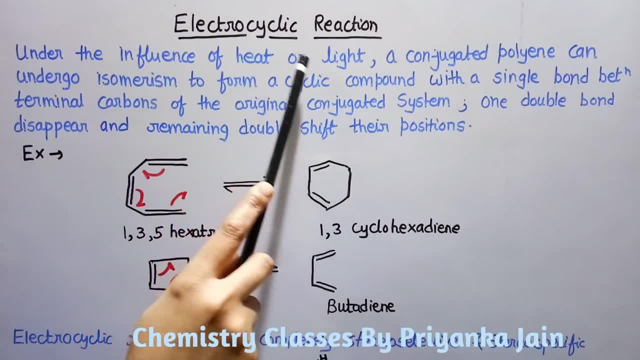 may undergo when it is exposed to heat or to the light. It may undergo isomerism to form a cyclic compound And in this process a new sigma bond is formed at the expense of a double bond and the rest of the double bonds shifts their position. for example, if we see: 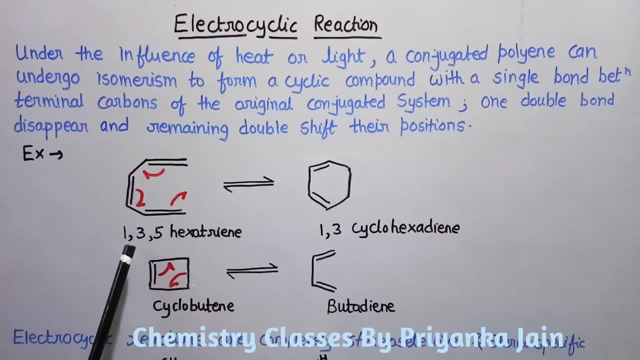 this example. this is a open-chain compound, that is, 135 hexadryene. it is a conjugated polyene system and when it is exposed to heat, which means when it undergoes a thermal or the photochemical cyclization, it forms one three cyclohexadirene, and in this process a new sigan bond is formed between this. 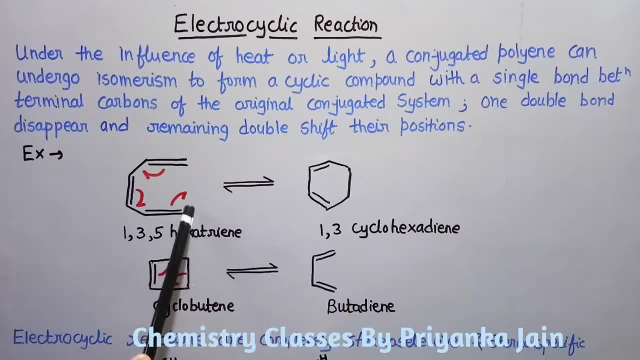 and this carbon atom. a new Sigma bond is forming between these two carbon atoms and here are three double bonds present, but one double one disappear and the rest of the double bonds will transfer their position so that the new compound possess a new Sigma bond and the two double bonds. so this type of process is 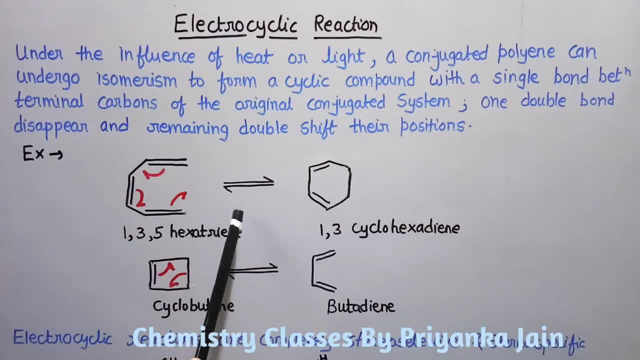 called the cycle H ancora as GRI L. there is bound process when a atom 같은�os electrocyclic reactions, and this is a reversible process. it means it may involve the ring closure or the ring opening. another example is the cyclobutene. when this compound undergoes the electrocyclic reaction under the 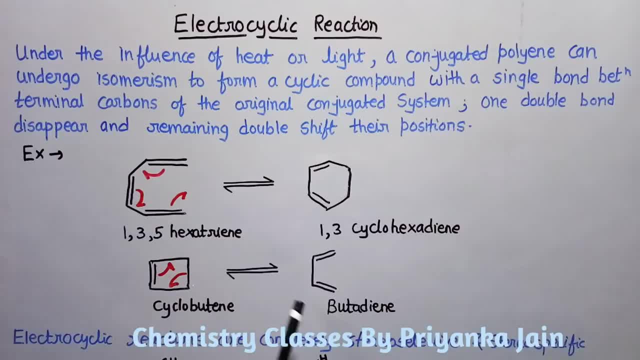 thermal or the photochemical conditions, it forms a new compound, open chain compound, that is butadiene. this is a ring opening process. I have shown here the reversible process. that is the ring opening. here a sigma bond is present and this sigma bond disappears, a pi bond is forming. so here two pi bonds are present. 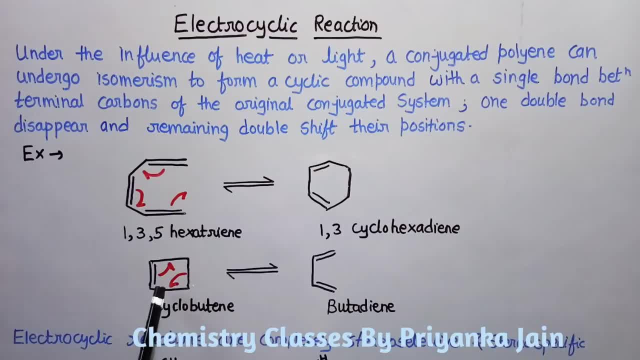 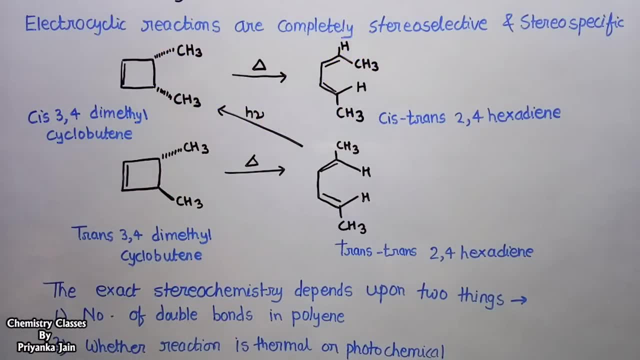 and the Sigma bond is disappear. so the cyclic compound is changing to a open chain compound. the electrocyclic reactions are completely stereoselective and stereospecific. what is meant? it means that a specific job is performed and at some stage, the person behind the computer is the one. 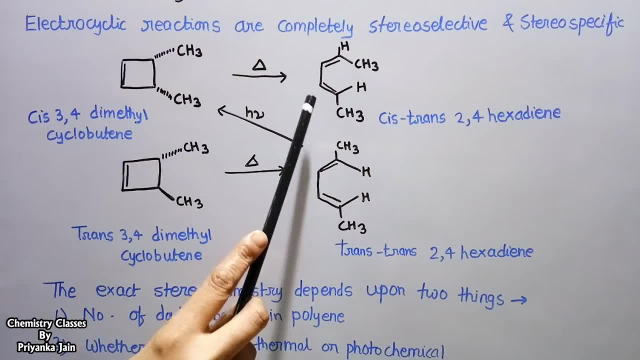 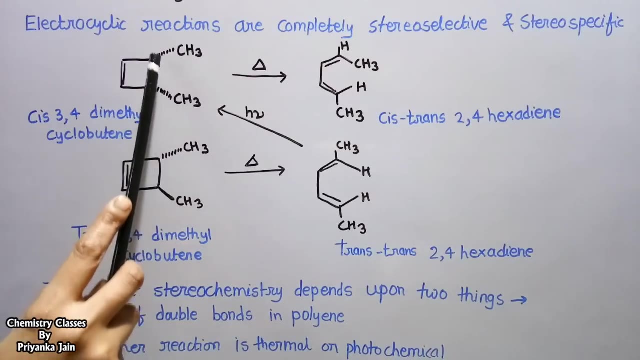 geometrical isomer gives rise to a specific geometrical product, while the another geometrical isomer gives to the different product. such type of reactions are called stereospecific reaction. for example, this is cis 3- 4 dimethyl cyclobutene. in this compound, the two methyl groups, both are 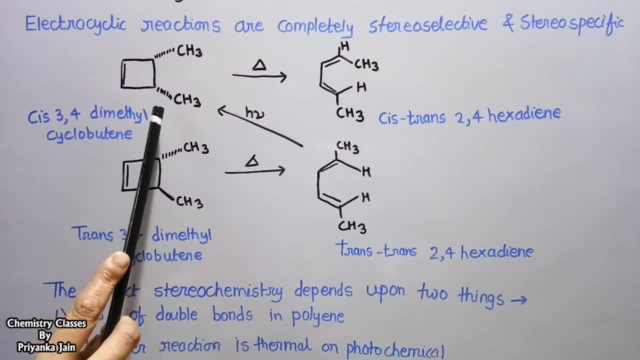 below the plane. so it is a cis geometry. and when it is, when it undergoes the electrocyclic reaction- thermal under thermal conditions- it forms the product that is cis trans product. this is a cis trans product because this methyl group is here and where the anodar is in the different position. 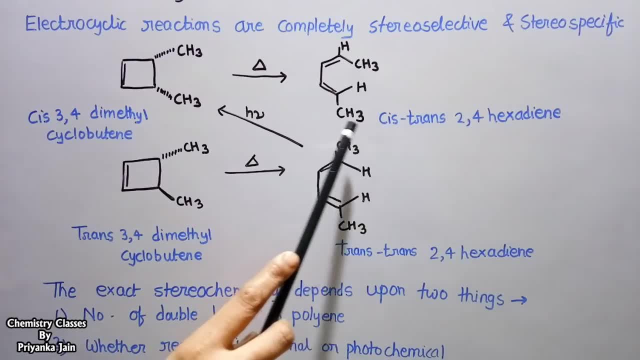 not cis position. one is cis and another is trans, so this is called a cis trans position. so this product gives rise to the cis trans product, while this is a trans 3- 4 dimethylcyclobutene. in this, one methyl group gives rise to the cis trans product and one methyl group gives rise to the. 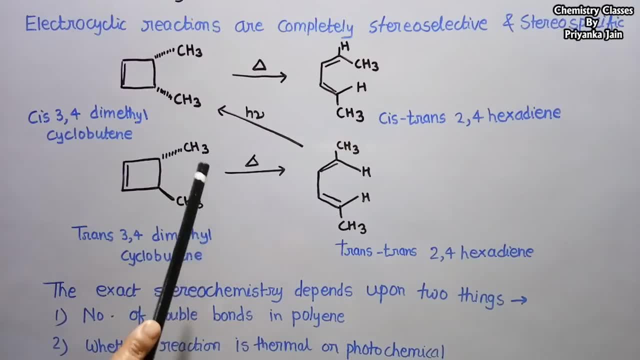 is below the plane and another is above the plane, and when it undergoes the thermal ring opening it forms the trans trans product. so these type of reactions are called the symmetry allowed processes and this product can give rise to when it undergoes the ring closer under the photochemical conditions. it 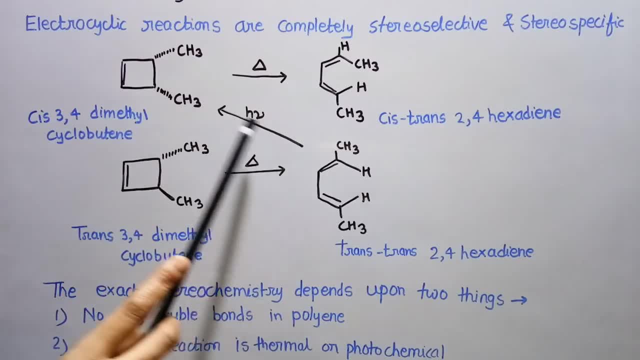 give rise to this type of product and this is also symmetry allowed. but it cannot be upon that this compound thermally gives this, that will be symmetry forbidden. so these reactions proceeds in the specific directions. the exact stereochemistry depends upon the two things. the first thing is the number. 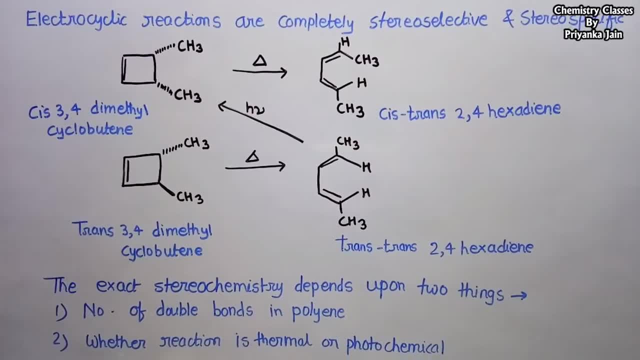 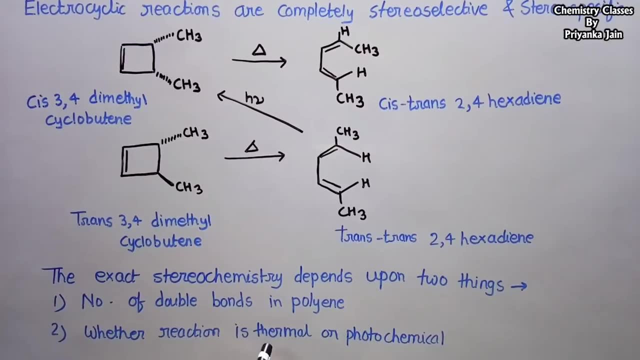 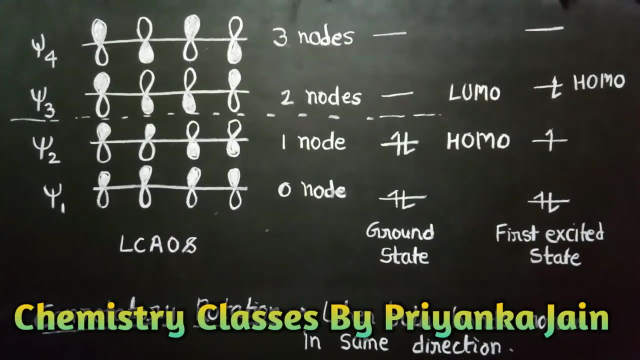 of the double bonds in the polyenes. and another condition is whether the reaction is thermal or the photochemical, because in both the conditions we get the different products. So in order to understand the symmetry allowed and trusting the symmetry forbidden process and what will be the stereochemistry of the product, we will 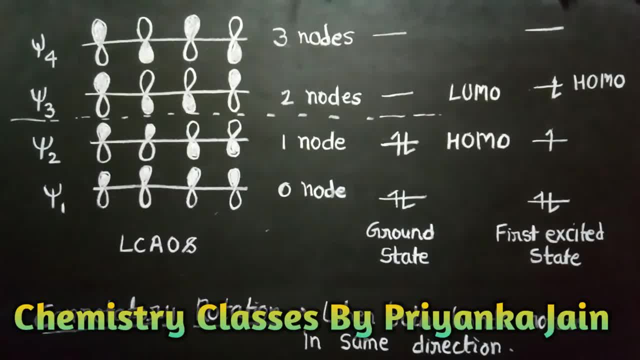 have to firstly understand what is the frontier molecular orbitals. if we see the case of the Buta diene, in this case there are 4 pi electrons present and in this case, if we see the linear combination of the atomic orbitals, there are four linear combinations. 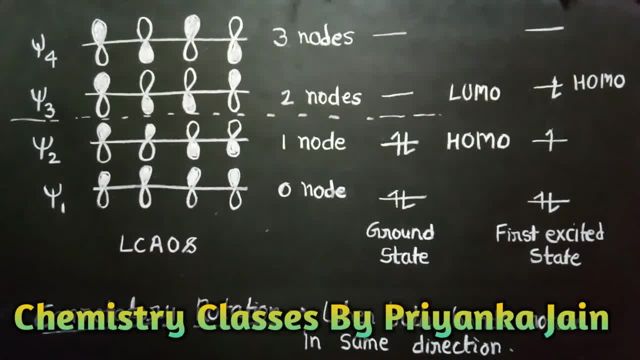 of the atomic orbital Psi 1, Psi 2, Psi 3 and Psi 4. these are in the increasing order of the energy. it means the Psi 1 will have the lowest energy, while the Psi 4 will have the highest energy and, in the case of Psi 1, all the orbitals. 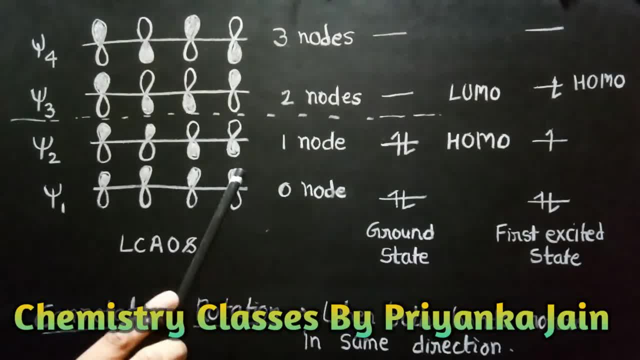 will have the same symmetry. and there is no node, it means zero node. in the Psi 2 there is one node present. these two have same symmetry and these two have the same symmetry, there is a node, so it will possess one node, while in the Psi 3, 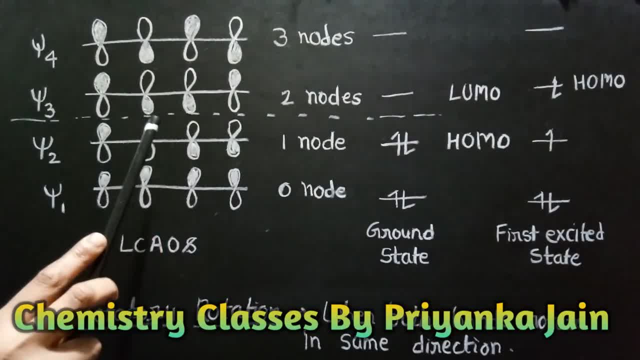 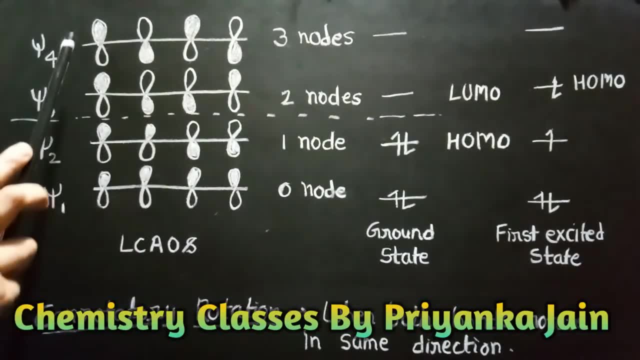 there are two nodes, 1, and the two nodes are present, and in the Psi 4 there are three nodes present. 1, 2 and 3 nodes are present in the case of Psi 4. these two are the antibonding molecular orbitals and these are the bonding molecular 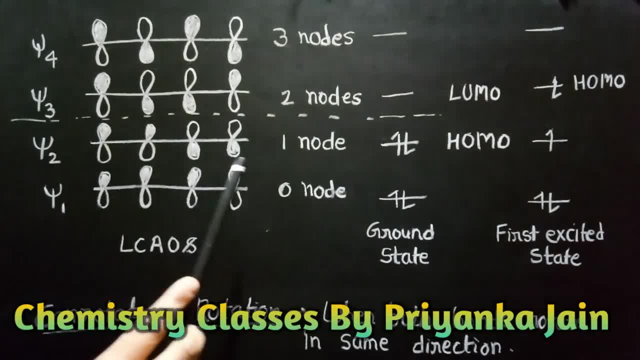 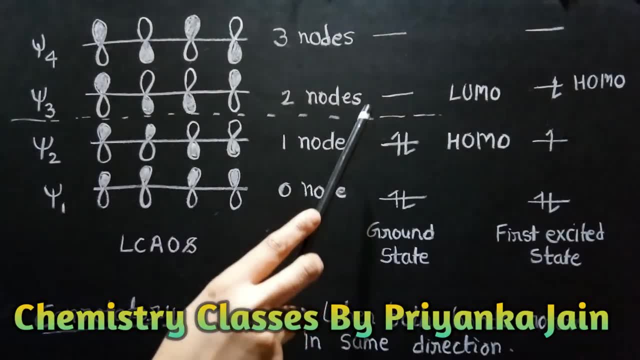 orbitals. so we see that four electrons to will in this orbital and to another will that in the Psi 2, Psi 1 and Psi 2 are failed, while the these two are the vacants. so we see, in this case, in the case of the, 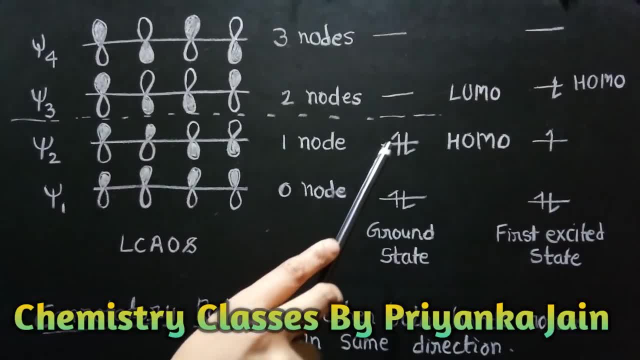 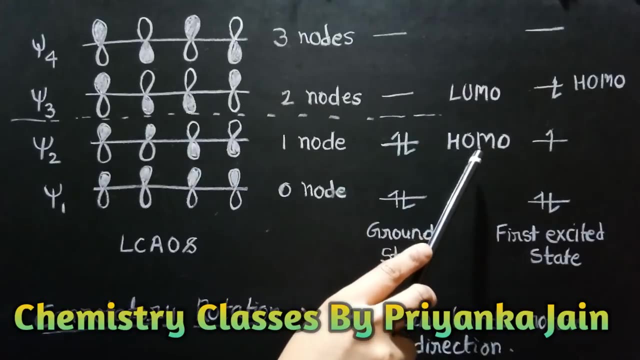 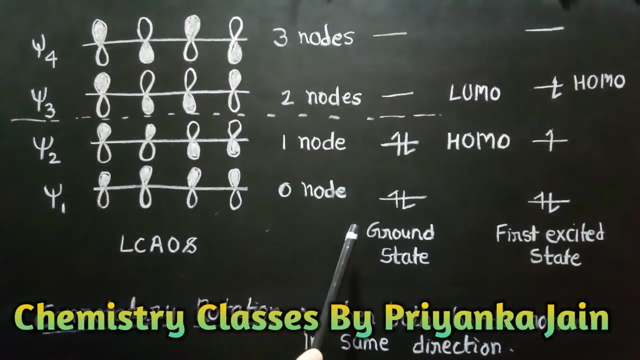 pericyclic reactions or the concerted reactions, we see the electrons in the highest occupied molecular orbital and that, in the case of this, butadiene, is the psi 2 orbital, that is the highest occupied molecular orbital, and this is the lowest unoccupied molecular orbital, that is psi 3, and this is the condition. 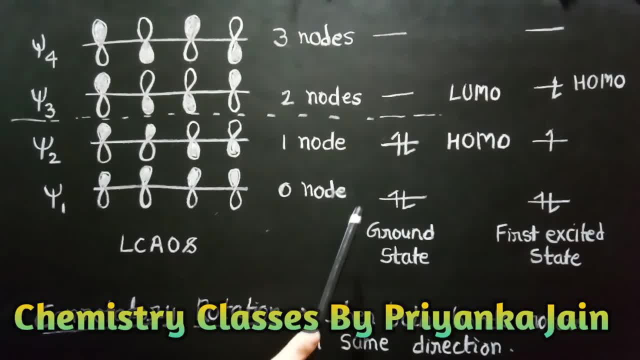 when the molecule is present in the ground state. but in the case of first excited state or when we see the photochemical process, when the reaction happens by the exposure to the light, then the molecule under will go to the first excited state. it means the one electron will jump from this orbital. 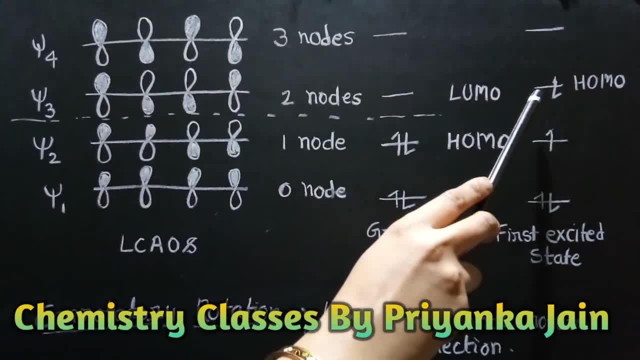 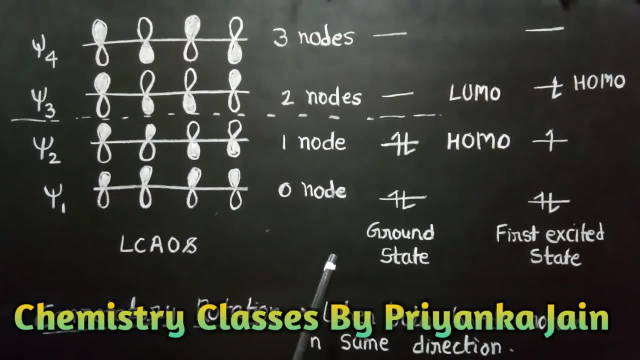 that is psi 2 to the psi 3. so now the electron one electron is present in this psi 3 orbital. so now the highest occupied molecular orbital will be the psi 3. so this thing should be very well cleared, because this is the thing that decide the geometry of the 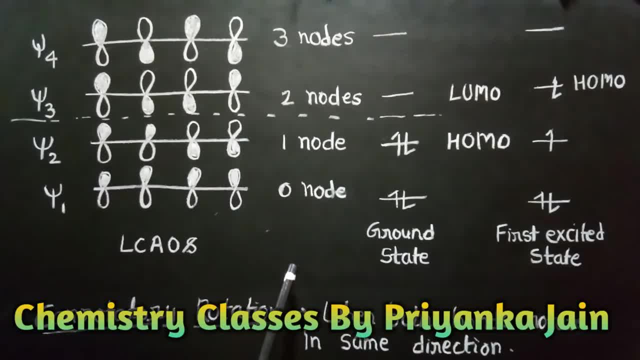 molecule. that is the highest occupied molecular orbital symmetry. and when we see the ring closer, what happens? we see the c1 and the c4 carbon atom. it means this and this carbon atom, this carbon atom and this carbon atom. we should have to see the symmetry of the orbitals at the c1 and the c4 carbon atoms in this. 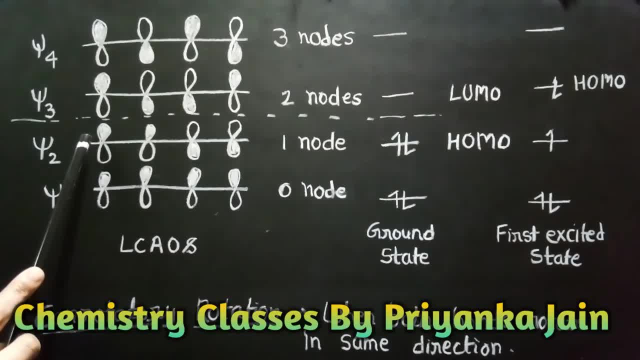 case, the highest occupied molecular orbital is psi 2 and we see the geometry of this and this and this will have the opposite. geometry is opposite. symmetry is present in these two orbitals because these two takes part in the formation of the sigma bond, because the present in the highest occupied molecular orbitals are loosely bind and 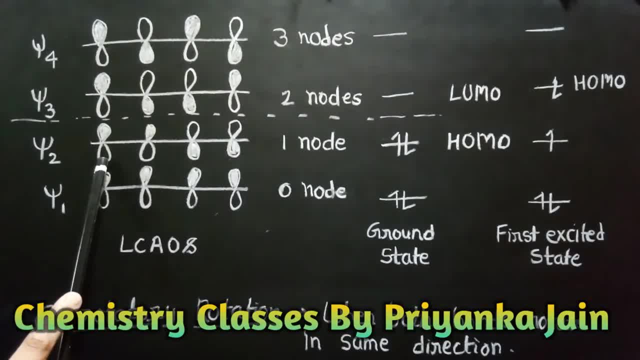 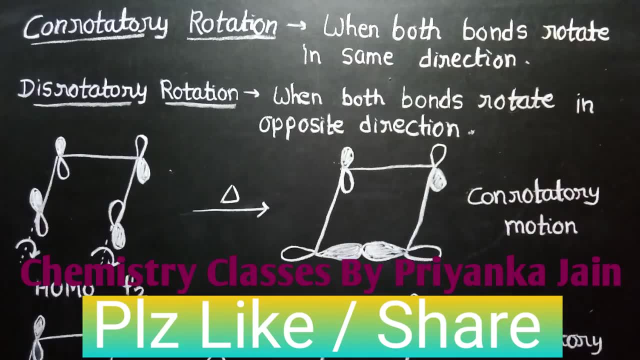 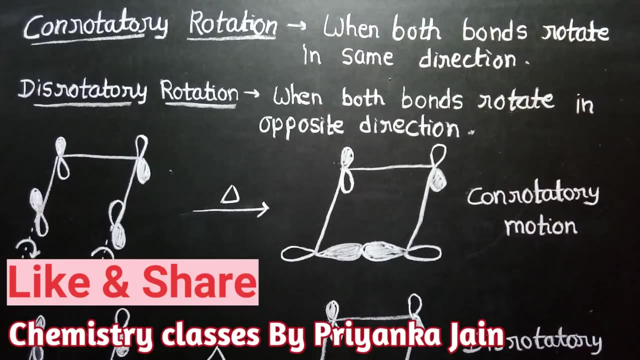 these two orbital will take part in the formation of the Sigma one. so we will have to see the geometry of these two orbitals for the ring closer, the overlapping between the terminal carbon atoms, the orbitals, the orbitals present at the terminal carbon atoms, should takes place, and for the better overlapping. 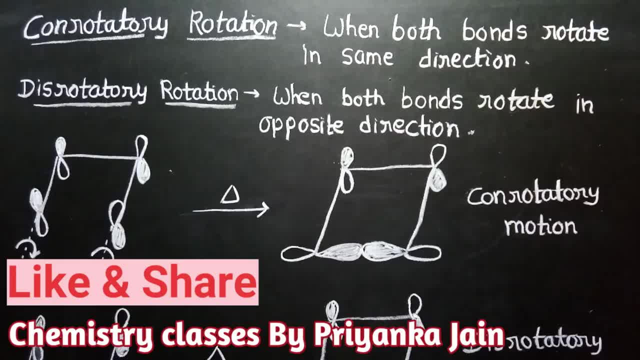 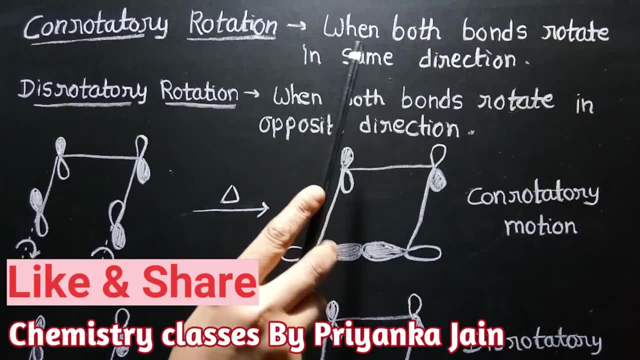 these orbitals should rotate and the rotation may be of two types. one is the come rotate- re rotation, when both the bonds rotate in the same direction. it means bonds rotate either anti-clockwise or both rotate in the clockwise direction. and another type is the disparity rotation. it means when 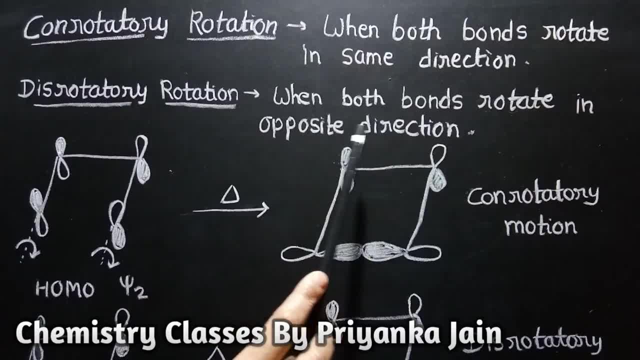 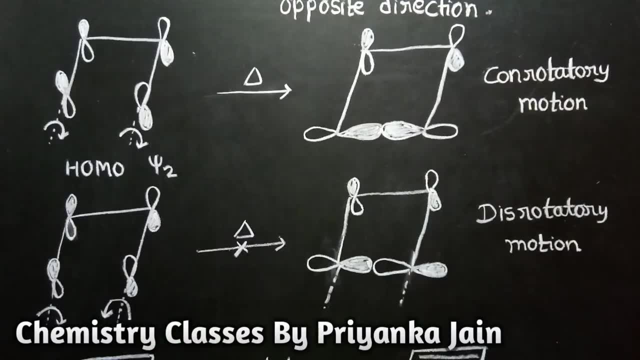 the both bonds rotate in the opposite direction: one rotates in the clockwise direction and another in the anti-clockwise direction. we can better understand it with the help of the example, as we know that the electro cyclic reactions can be carried out by the heat or by the light. 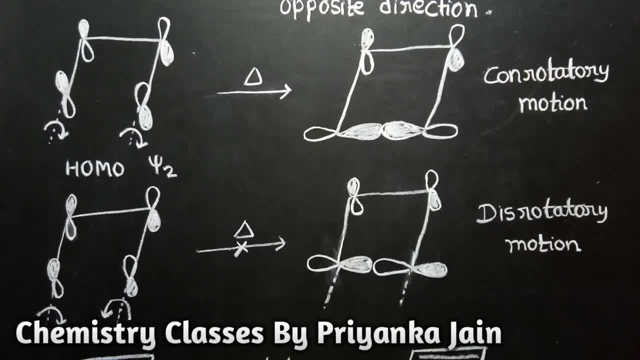 so, firstly, we see that thermal cyclization, thermal ring closure of the butadiene, in this case, the first condition is that we carry out the cone rotatory rotation. it means when we rotate both the bonds in the same direction. it means both the clockwise direction. so what happens? this lobe will. 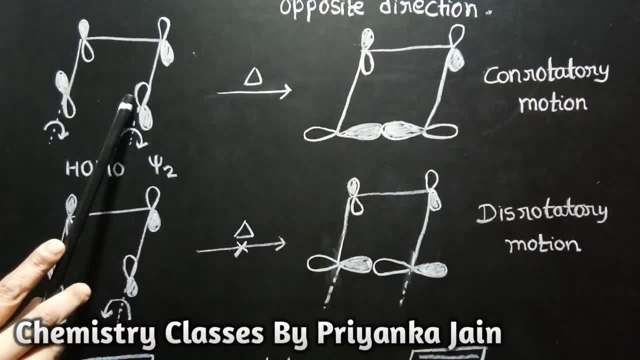 come here and this lobe will come here and this will come there. so such type of symmetry we get and this symmetry is better for the overlapping and in this condition a Sigma bond can be formed. so this rotate, this ring closer will be symmetry allowed and this will takes. this reaction will takes place because 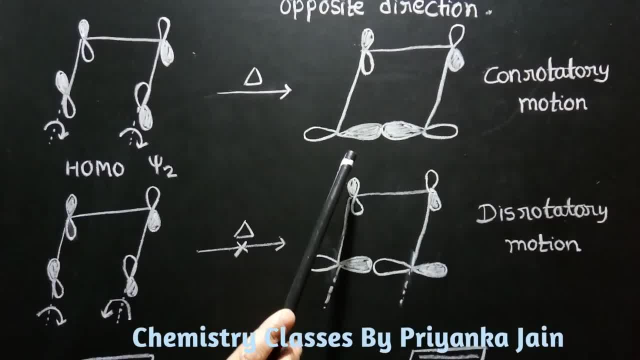 in this case a good Sigma bond can be formed. so this process is thermally allowed process and such type of rotation is called the cone rotatory motion. another condition is if we carry out the rotation, this rotatory, it means we rotate both the bonds in different direction, opposite direction, one anti clockwise and another. 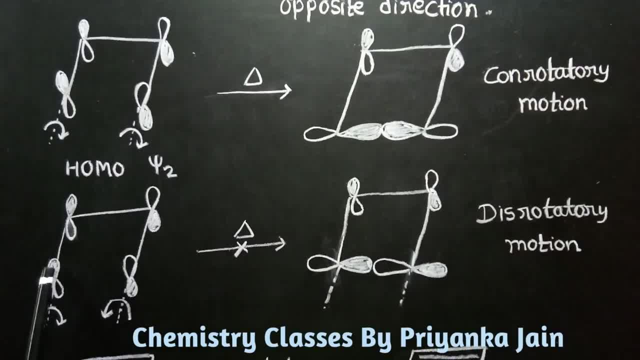 anti-clockwise. so what will happen? this bond will this lobe come here and this loop will come here. so we get a opposite symmetry and this symmetry is not good for the overlapping and no Sigma bond will be formed. so such a process in the case of butadiene is thermally forbidden. it will not happen. 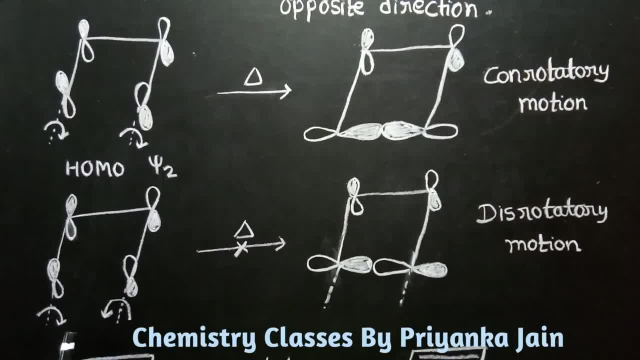 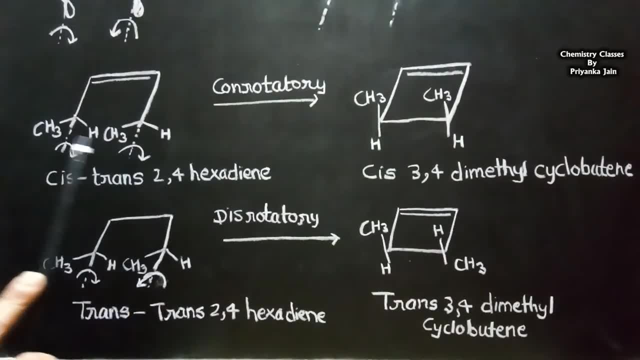 and this type of motion is called the this rotatory motion. now we see it with the help of the example. for example, if we see cis, trans 2, 4 hexadiene and it's two bonds, undergoes the cone rotatory motions. it means both are rotating in. 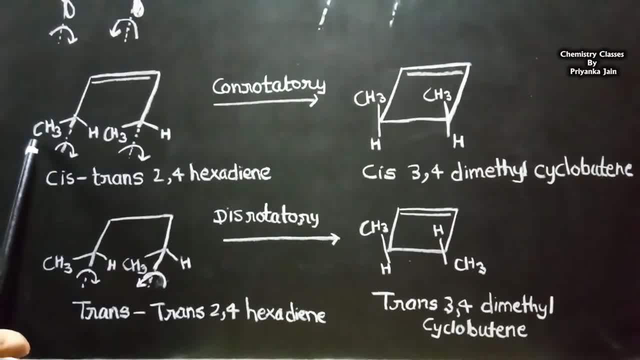 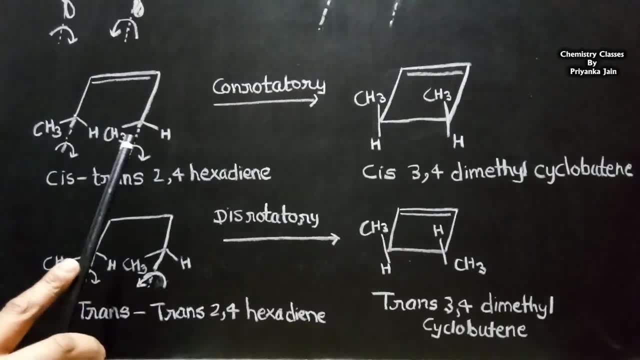 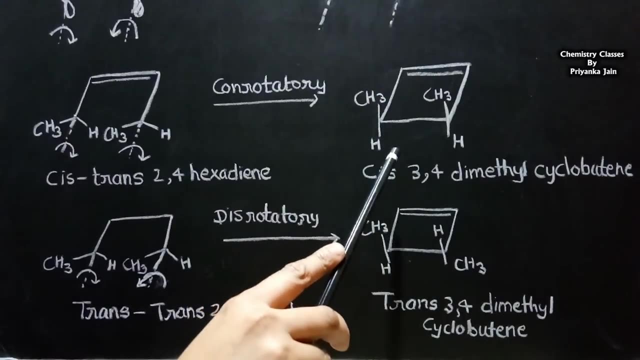 the same direction. or we can say clockwise what happens this methyl groups come above and this hydrogen goes below. this methyl groups come above and this hydrogen goes below, so we get the cis product. it means both the methyl groups are above the plane and both the hydrogens are below the plane, so we get 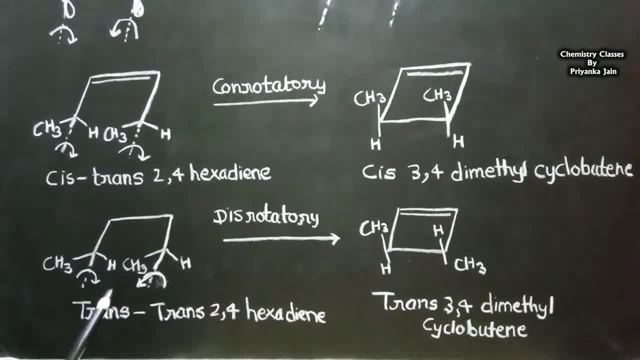 the cis 3, 4 dimethyl cyclo butane. similarly, we see the another product that is similarly. we see the cis 3: 4 dimethyl cyclo butane. that is similarly. we see the another compound that is trans trans 2, 4 hexadiene, and in this 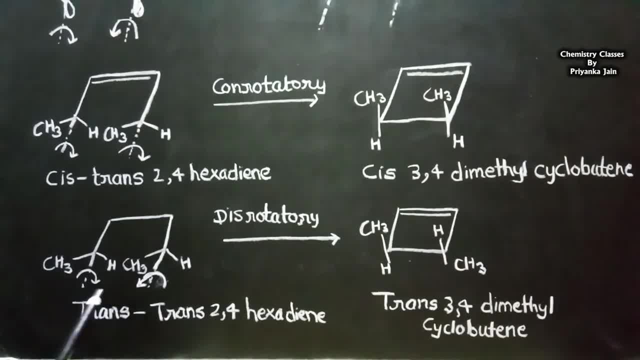 compound if the bonds are rotated in the reverse direction- opposite direction, it means when it undergoes that this rotate 3 motion- one bond is rotating clockwise and another is rotating anticlockwise- this methyl group will come above the plane. this hydrogen goes below, while this hydrogen comes above the plane and this methyl group goes below. this tables comes above, above the plane, and this methyl group goes below. 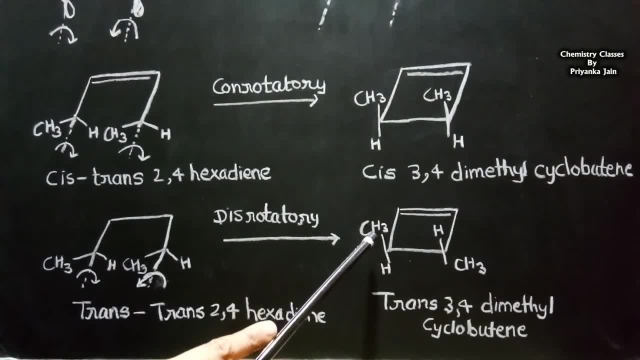 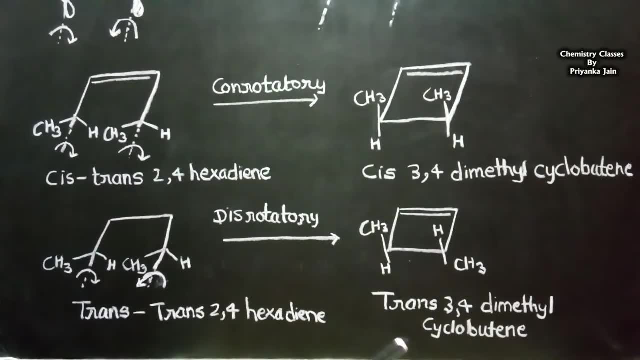 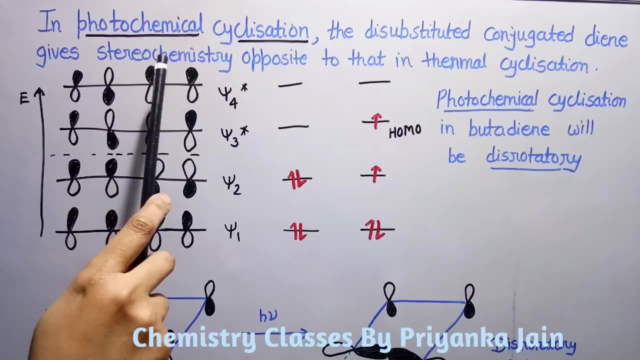 So we get a trans product. It means one methyl is above the plane and another methyl is below the plane. So we get trans 3,4-dimethylcycloputene. Photochemical cyclization: The disubstituted conjugated diene gives stereochemistry, opposite to that in the thermal cyclization. 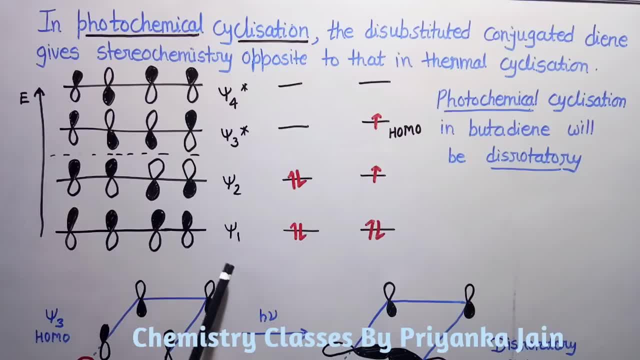 For example, if we see the linear combinations of atomic orbitals of butadiene, As we have said earlier that in the ground state the electrons are occupied in these two orbitals, It means the highest occupied molecular orbital is psi 2 in the ground state, That is, in the case of thermal cyclization. 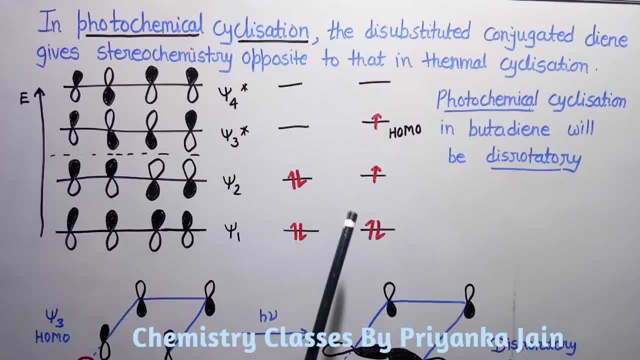 But in the case of photochemical cyclization what happens? As a result of the light, the one electron is promoted further From this orbital to the psi 3 orbital. Now the highest occupied molecular orbital becomes this psi 3.. So you can see, in this case, the two orbitals that are the terminal carbon atoms, that are attached to the terminal carbon atoms. 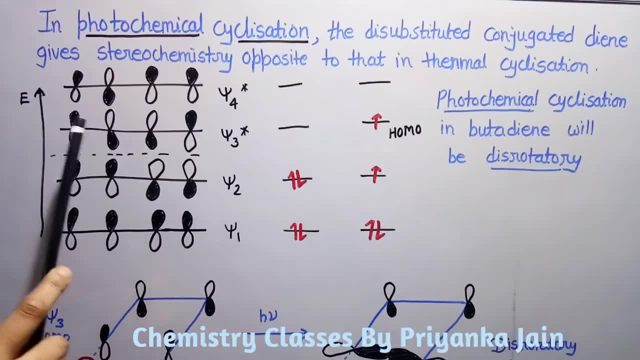 These two orbitals have the opposite symmetry, But in this case these two have the same symmetry, So the condition becomes different. In this case the Disrotatory rotation will give a formation of the sigma bond. So the photochemical cyclization, in the case of butadiene, will be disrotatory. 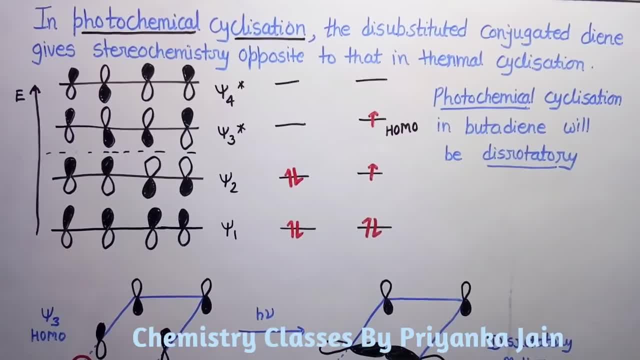 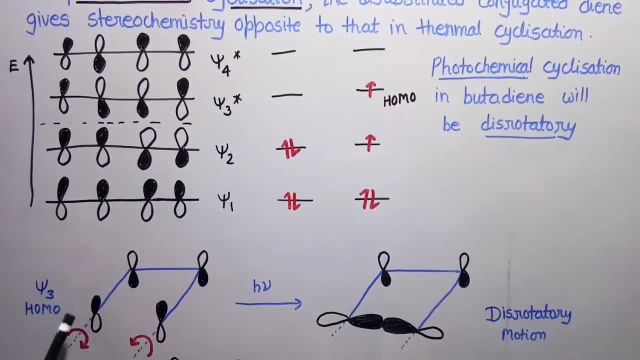 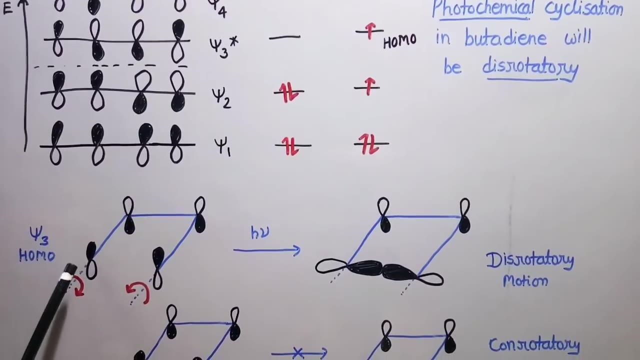 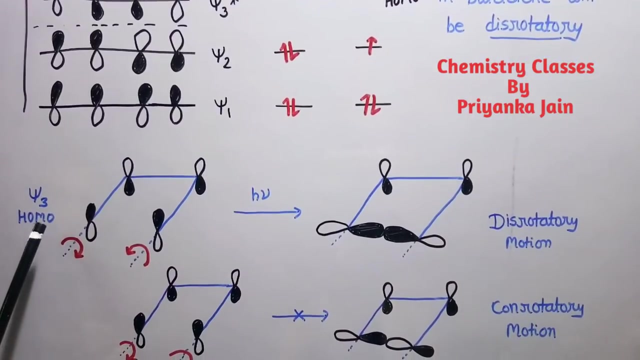 You can see it with the help of this example. This is the highest occupied molecular orbital In the case of first excited state, or we can say, in the case of photochemical cyclization, When one electron has Been promoted to the psi 3 orbital and this has been become the highest occupied molecular orbital. 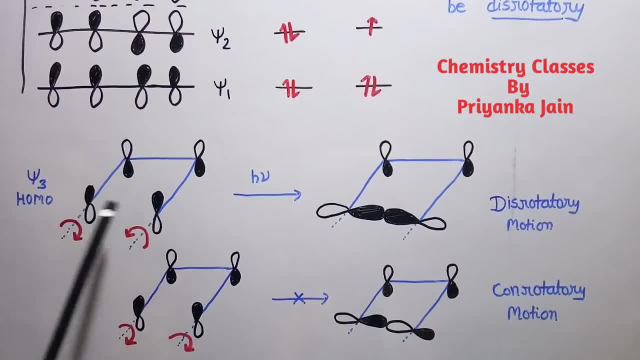 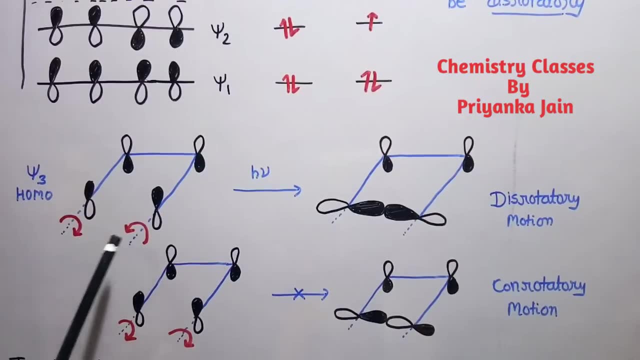 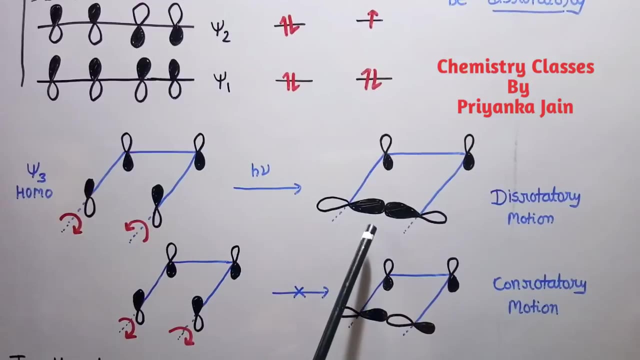 So we have said that the two terminal orbitals will have the same symmetry. So the disrotatory motion will give the sign of symmetry, the significant symmetry that is required for the formation of the sigma bond. This is the disrotatory motion. 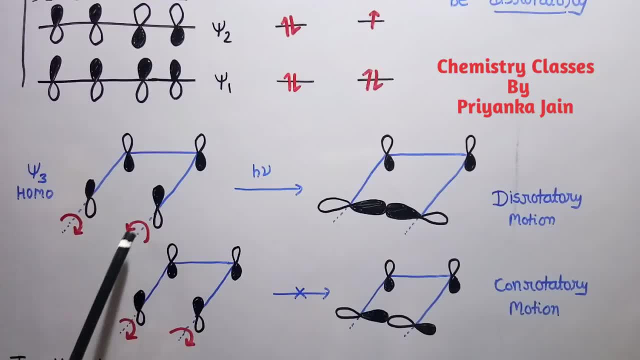 It means one is moving in the clockwise direction and another is moving in the anticlockwise direction. So the photochemical cyclization in the case of butadiene will be by the disrotatory motion. If we see the conrotatory motion, what will happen? 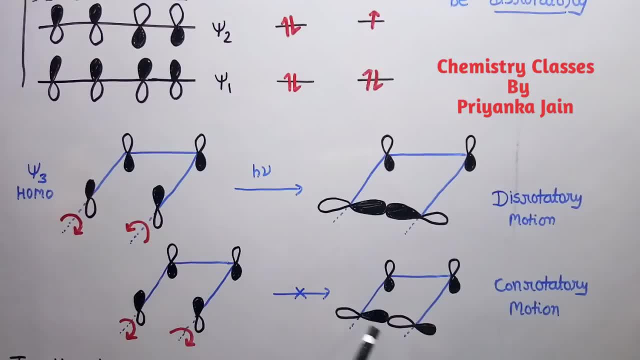 This will rotate here and this will also rotate here. So we get this type of symmetry. It means opposite symmetry, So it cannot form a sigma bond. So such type of reaction is symmetry forbidden. The only symmetry allowed state in the case of photochemical cyclization will be by the disrotatory motion. 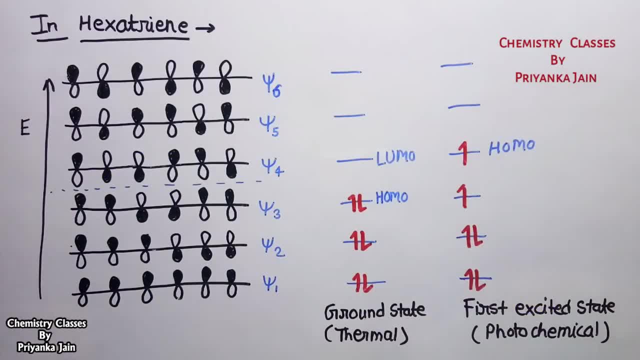 We have seen here the electrocyclic reactions for the 4N system, that is, the butadiene. Now we see the electrocyclic reaction for the 4N plus 2 system. An example of it is the hexadrine. 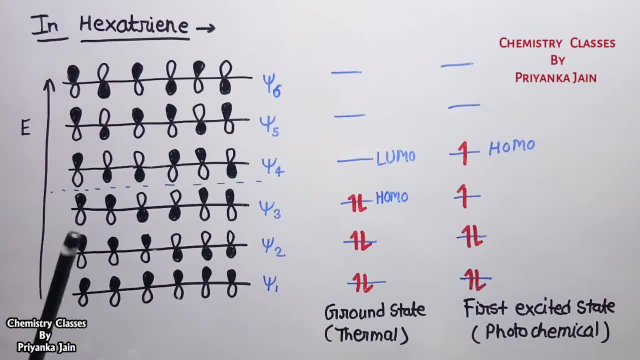 In the case of hexadrine, the linear combination of the atomic orbitals, there are six combinations, That are psi 1, psi 2, psi 3, psi 4, psi 5 and psi 6.. And if we see their symmetry properties, in this case all the orbitals are symmetric and there is no node. 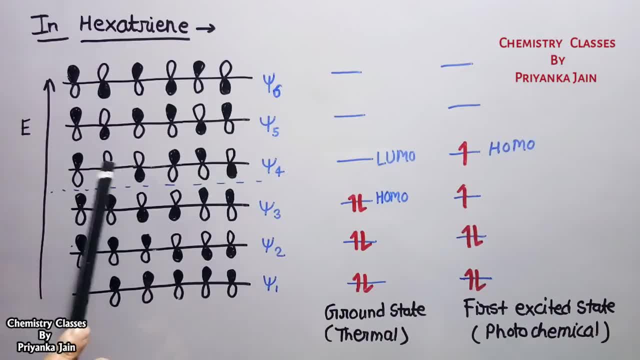 There is one node, there are two nodes, there are three nodes present And here are four, and here five nodes are present And these three are called the bonding molecular orbitals, while these three are the anti-bonding molecular orbitals. So electron will fill according to the increasing energy. 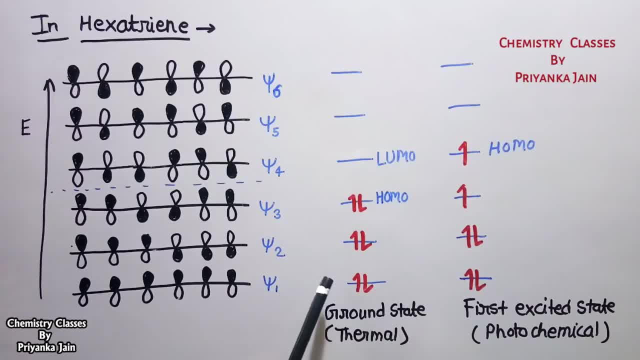 It means it will fill in the three bonding molecular orbitals. So this is the highest occupied molecular orbital and this is the lowest unoccupied molecular orbital. So in the case of the ground state, that is important in the thermal cyclization. 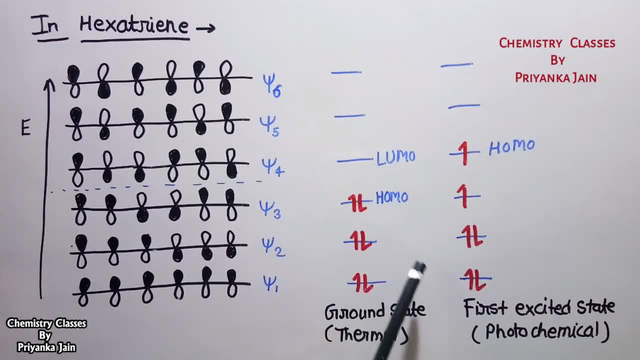 The psi 3 is the highest occupied molecular orbital, While if we see the first excited state that is important in the photochemical process, photochemical cyclization, When we expose a molecule to the light, what happens? One electron is excited from this orbital to the psi 4 orbital. 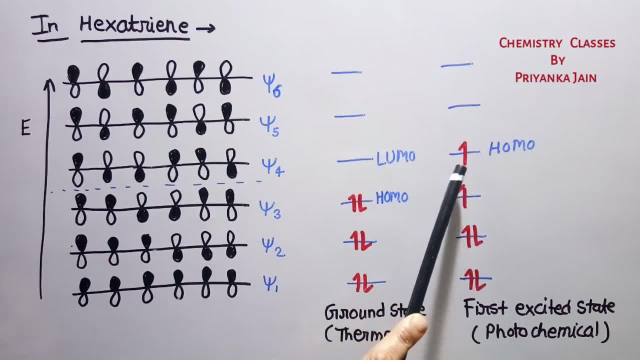 So what happens? This psi 4 will become the highest occupied molecular orbital. So, according to the frontier molecular orbital concept, this is very important in the case of pericyclic reaction. These highest occupied molecular orbital and the lowest unoccupied molecular orbitals are very important thing. 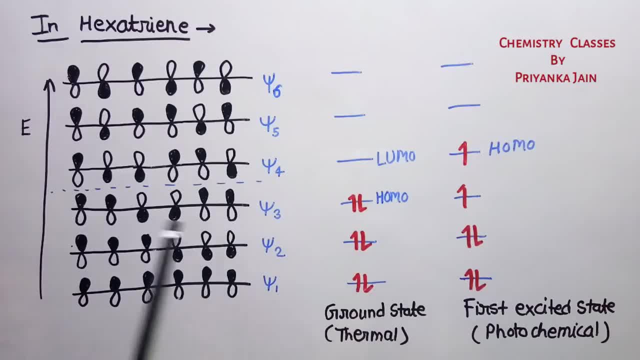 We should remember them, So we should see the symmetry of them. In this case, for the thermal cyclization, we can see, the terminal orbitals will have the same symmetry, While for the photochemical cyclization, these terminal orbitals will have the opposite symmetry. 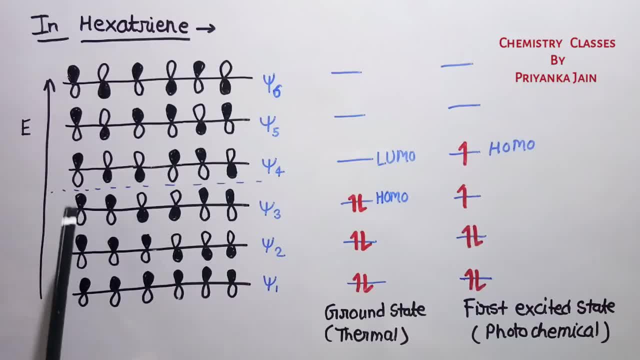 So in the case of thermal cyclization, the dis-rotatory motion will take place, While in the case of photochemical cyclization, cone-rotatory motion will take place. We can see the symmetry property with the help of the example. 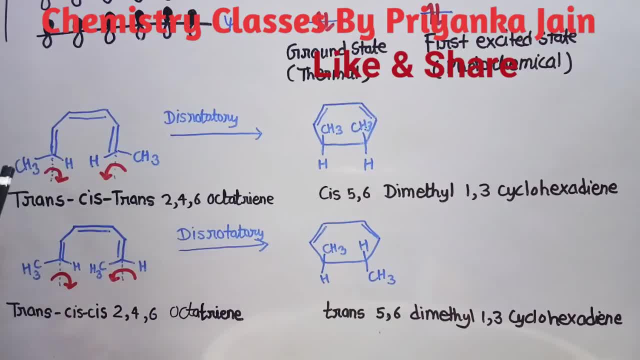 This is trans-ris-trans-2,4,6-octa-triene, And here the two methyl groups are outside, while two hydrogen groups are inward. So in this case, if the dis-rotatory motion takes place, what will happen? 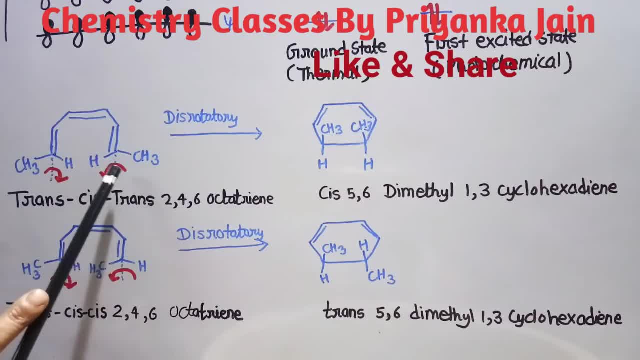 This bond moves clockwise, while this bond moves anticlockwise. So this methyl group comes above the plane, while this methyl group also comes above the plane And these hydrogens go below the plane. So we get this molecule, This molecule in which both the methyl groups are above the plane and both the hydrogens are below the plane. 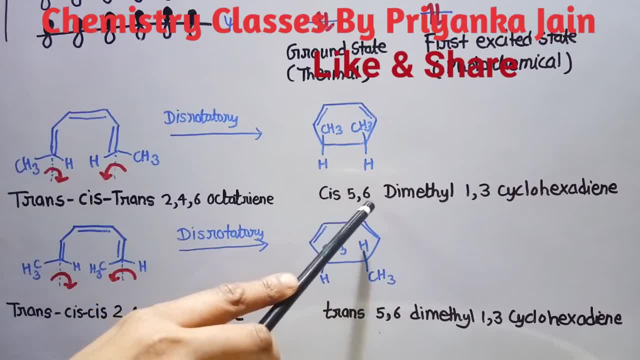 So this is a cis geometry And this molecule is cis-5,6-dimethyl-1,3-cyclohexadiene. Similarly, if we see the another molecule that is the geometrical isomer of this molecule, 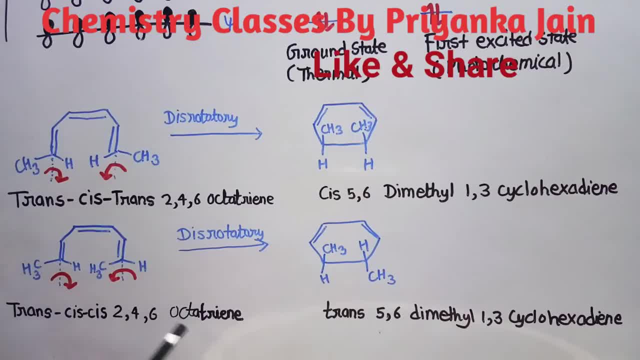 that is, trans-cis-cis-2,4,6-octa-triene. In this molecule the one methyl group is outside and another is inside, And if we carry out the dis-rotatory motion, the one bond will move clockwise and another rotates anticlockwise. 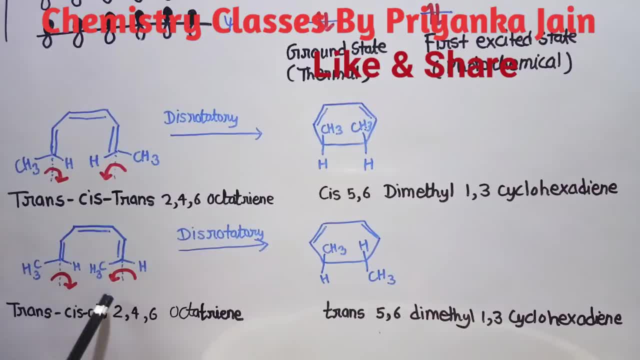 So this methyl group comes above and this methyl goes below the plane. So we get a molecule in which this methyl group is above the plane and this methyl group is below the plane And we get a trans-rheumatoid And the molecule will be trans-5,6-dimethyl-1,3-cyclohexadiene. 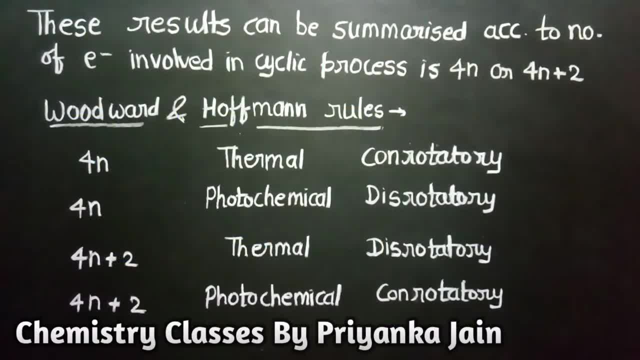 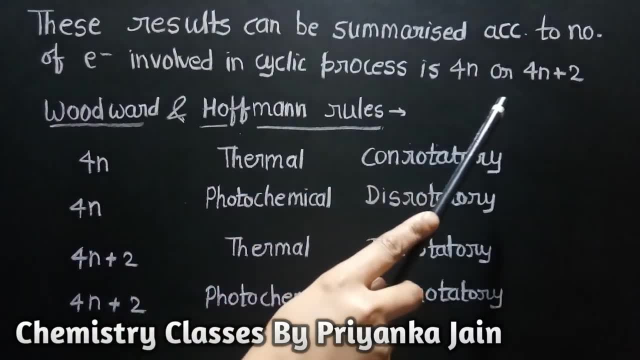 And the molecule will be trans-5,6-dimethyl-1,3-cyclohexadiene. These results can be summarized according to the number of the electrons involved in the cyclic process, Whether it is 4n or 4n plus 2.. 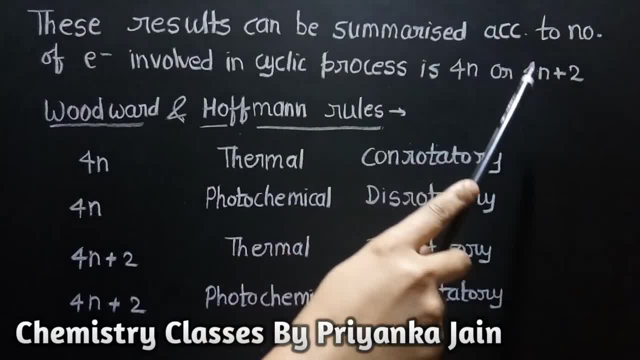 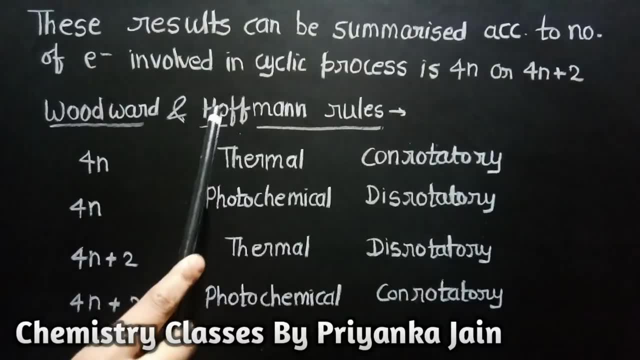 Because this will decide whether the electrons are 4n or 4n plus 2.. It will decide the symmetry of the electro-cyclic reactions And this is given by the Boudward and Hoffman's rule, For example, in the case of 4n system. the example of it is butadiene. 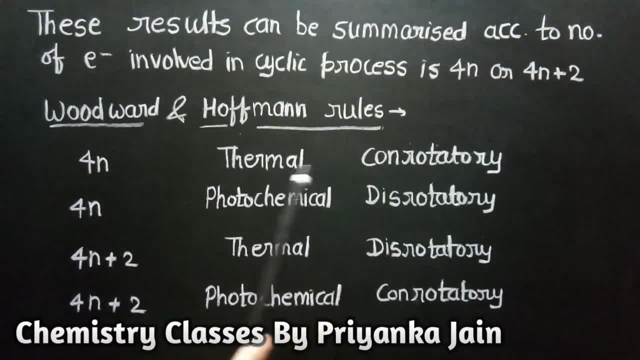 In the 4n system, the thermal process process. In the case of 4n system, the example of it is butadiene And the thermal process process, While the photochemical process processes by the disrotatory motion, While in the case of 4n plus 2, the thermal process processes by the disrotatory motion. 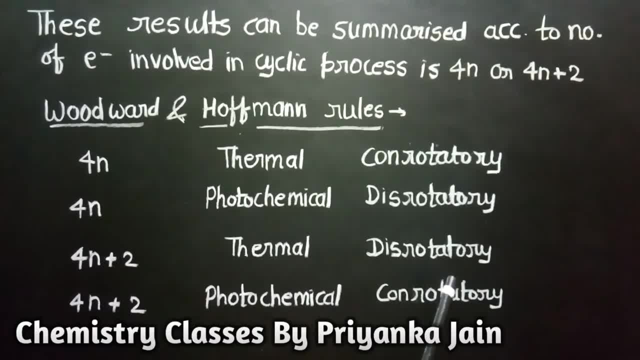 While the photochemical process processes by the cone rotatory motion. So if you remember any of these, you can get all of these, Because these are opposite to each other. For example, In the 4n, if the thermal process by cone rotatory 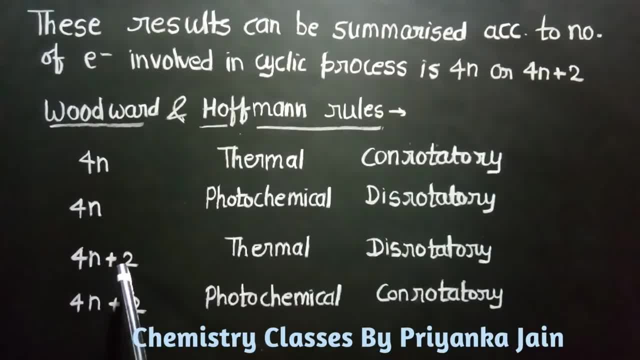 then the photochemical will be disrotatory. this rotatory similarly in the 4n plus 2. if the thermal proceeds by this rotatory, photochemical will be proceed by cone rotatory, similarly the 4n and 4n plus 2. 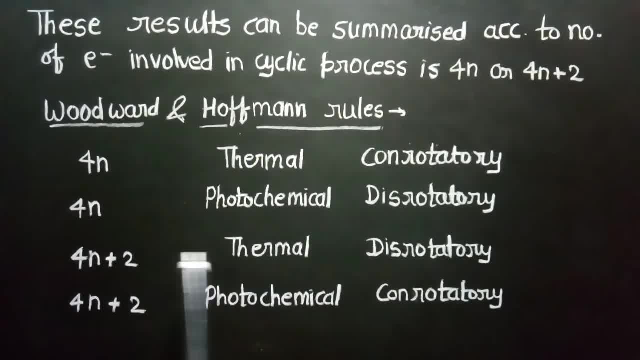 the thermal proceeds by cone rotatory, then the thermal in 4n plus 2 will proceed by the this rotatory motion and the example of this, the 4n plus 2, is the hexa trying. so this is all about the electro cyclic reactions in our next. 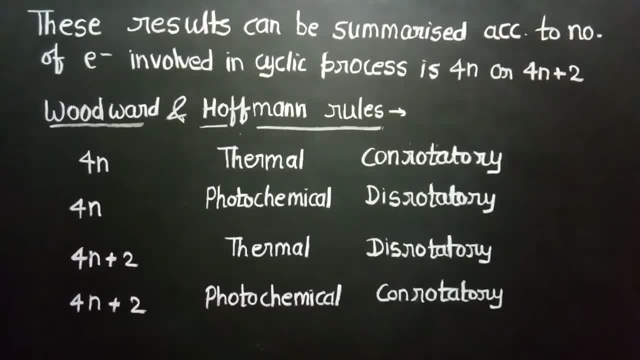 video we will understand about the cycloaddition reactions and all other type of pericyclic reactions. thank you. 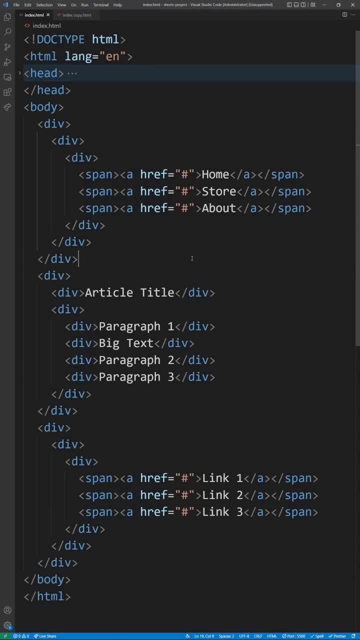 Here are three huge HTML mistakes I see most beginners making, and the first one is obviously not using semantic HTML. Everything in here you can see is divs and spans for the most part, which is confusing to read and difficult for screen readers to parse. Instead, your code. 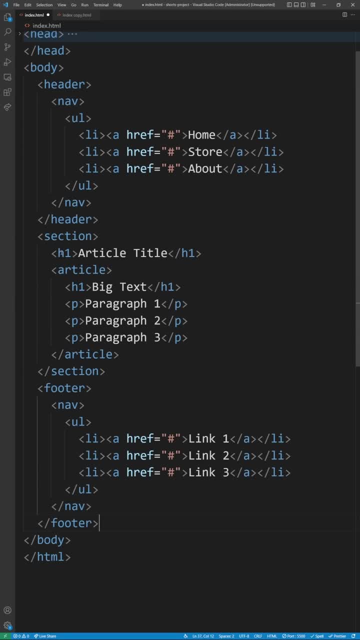 should look something like this: where you have headers, nav, ul, sections h1, articles, Everything that's defining what your content is is using these different semantic HTML elements. The second thing I see people making mistakes on all the time is not using the main element. 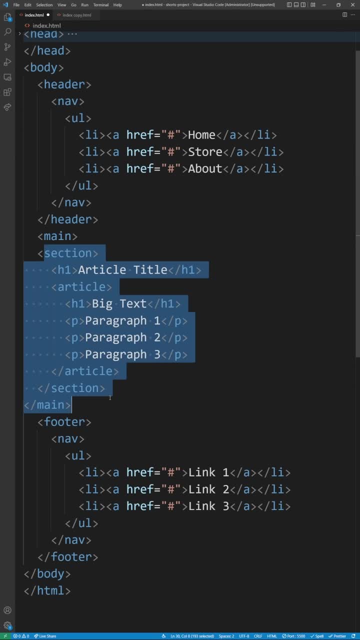 The main element just tells your browser what the main content in your article or page is. In our case, this section right here is our main content, so we're wrapping it in the main tag and you should only ever have one main tag- Another big mistake, speaking of one tag only. 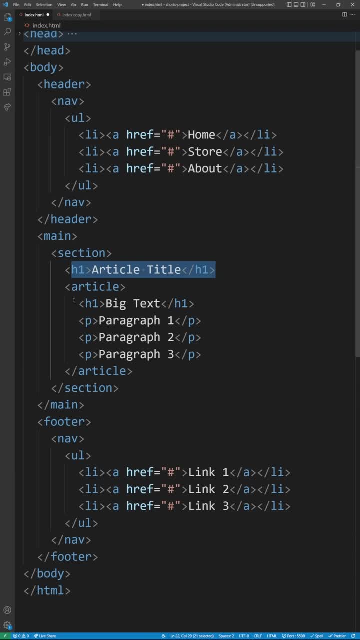 is h1s. You should only ever have one h1, and if you're using a heading element like an h1 just to make text big, instead you should replace this with something like a div or a span, and you should just give it a class that says something like big font, and that way it's not going to. 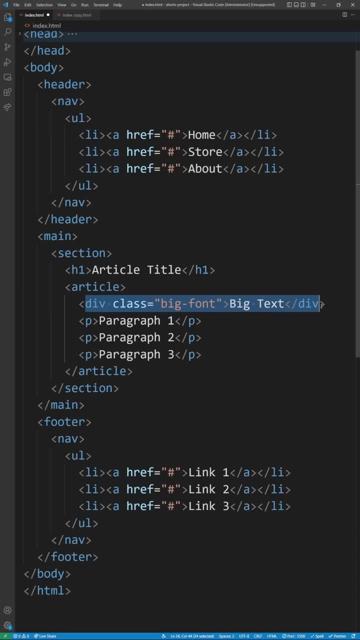 give any false meaning to the user. This is not a heading. this is just bigger than normal text.